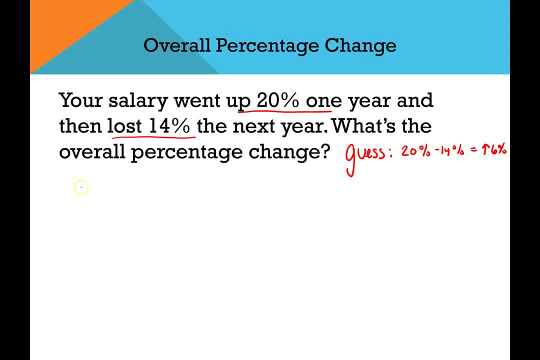 as a class, let's choose a number to start with, And let's always start with 100. And 100 is a pretty pathetic salary for the year, but let's just stick with 100.. So if I went up 20%, I'm going to go up 20%. And if you're saying hey, why the heck are you doing? 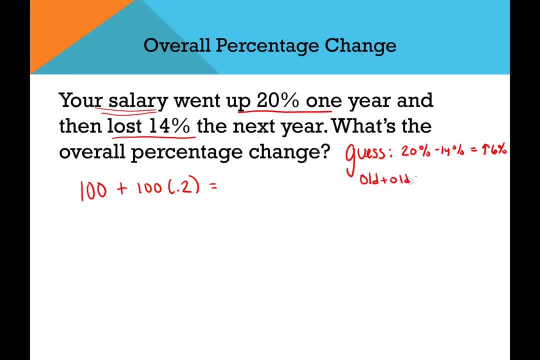 that That is old plus old. percent equals new. That's my 100 plus 100 times the percent increase is going to be my new value. Well, what is that going to be? That's going to be 100 plus 100 times the percent increase is going to be my new value. 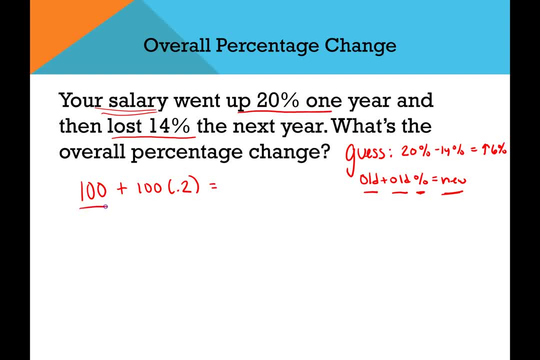 100 times 0.2 is 20.. So this is going to be: 100 plus 20 gives me 120. And you probably could have reasoned that out yourself. But now, the next year, you're going to take your $120 salary And 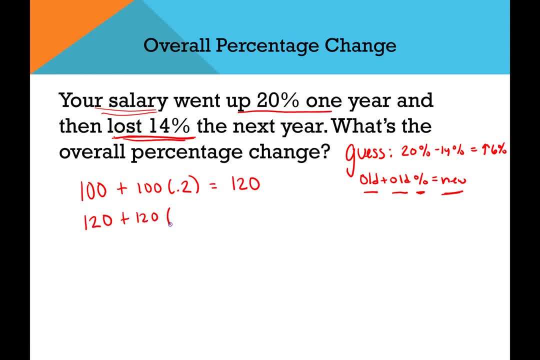 now you're going to lose 14%, So I'm going to have a negative 0.14 here. So this is old value from the previous year plus the old value from the previous year times. you've decreased 14%. So I'm going to have to throw that in my calculator And I get a 103.2. 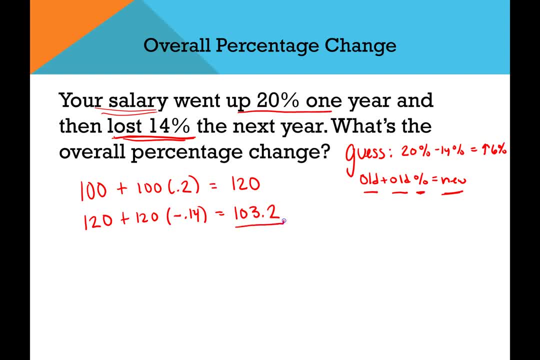 So how much has that gone up? Well, I have to take this 103.2 in my original value And I have to do new minus old over old. Well, this is my new salary And this is my old salary, So this is. 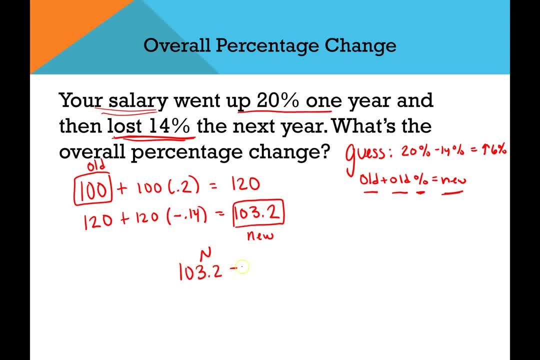 going to be 103.2.. My new minus my old of 100, all divided by old. So that's going to clearly give me 3.2 in my numerator. My old is 100.. So it's going to give me 3.2 divided by 100. 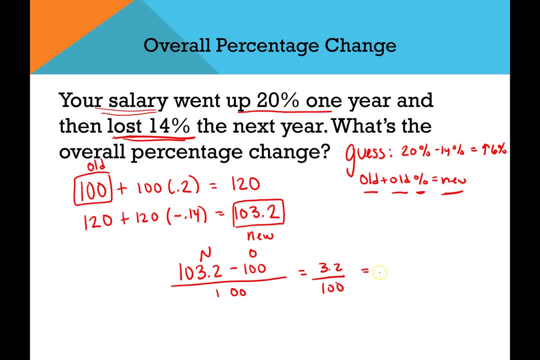 That gives me bringing the decimal back two places: 0.032.. And then we have to multiply by 100. And that gives me 0.032.. And then we have to multiply by 100. And that gives me 0.032.. And 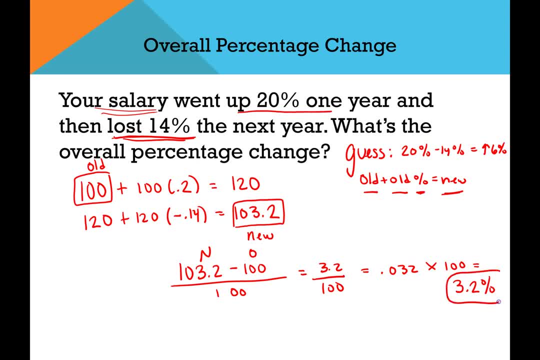 that gives me 3.2%. So you don't get 6% increase, you get 3.2% increase And that is going up 3.2%. I do want you to note- we've got some sort of a pattern here- that my answer was 3.2% And 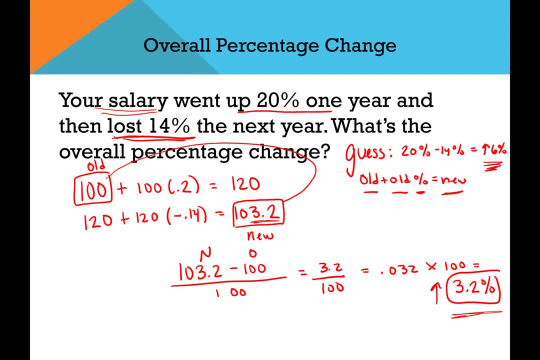 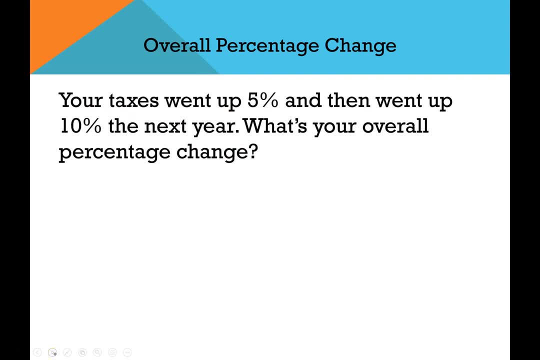 this is 3.2 bigger than 100.. I wonder if that pattern is going to continue. What do you think? All right, your taxes went up by 5% and then went up by 10% the next year. What's your? 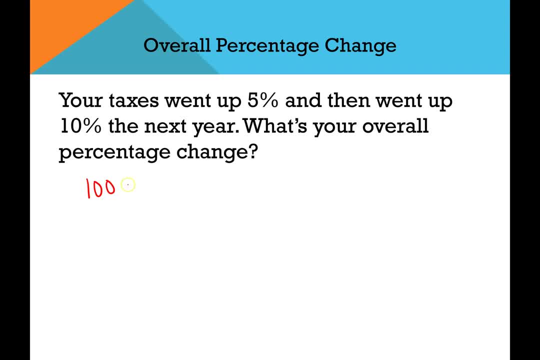 overall percentage change. Let's start with 100.. And then we've got went up. 5% is a 0.05.. So that's going to give me 100 plus 100 times 0.05.. That gives me 105.. Hopefully you did that. 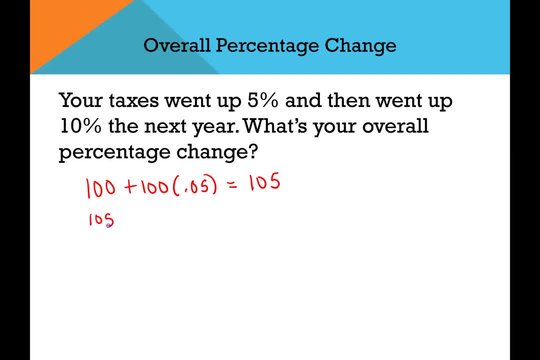 in your head. Now I need to take that 105. And I'm going to go up 10%, So that's going to be a positive 0.10.. So what does that give me? I'm just going to plop that right in And I get 115.5.. 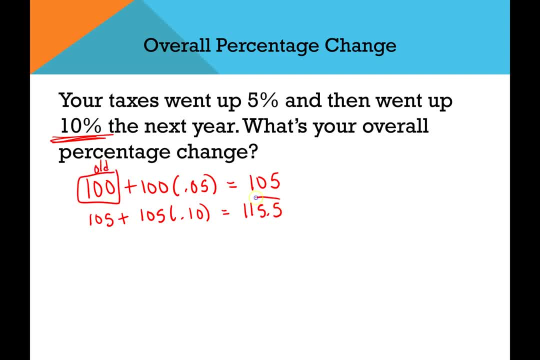 So here's my old, Here's my new salary, or taxes, my bad. Let's do new minus old over old. So this is 115.5 minus 100 over 100.. Well, that's going to give me a 15.5 divided. 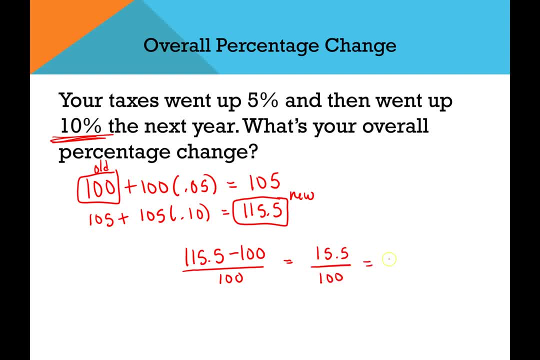 By 100. That means bring my decimal over two places. That's a 0.155.. Multiply by 100 and I get 15.5%. So it went up 15.5%. So you know, this is starting to make me feel like we really do. 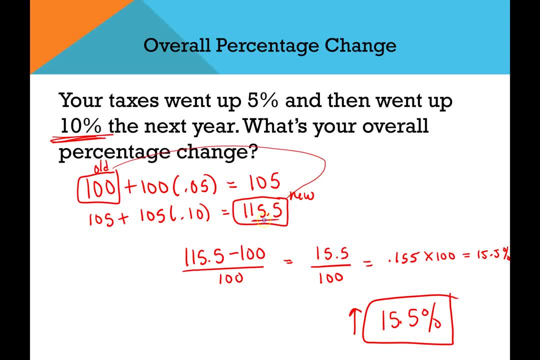 have a pattern that we're just going to take this answer- and it went up 15.5%. All right, What would have your guess been? Maybe before this class, you might have said it went up 15%, which is close, but it actually went. 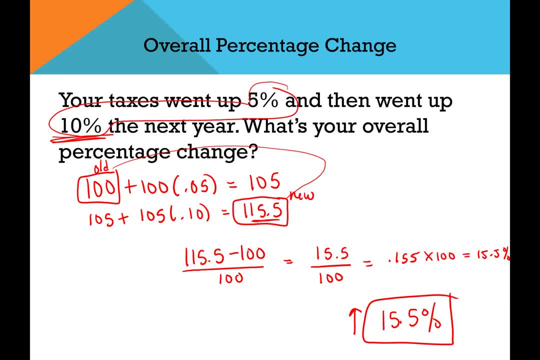 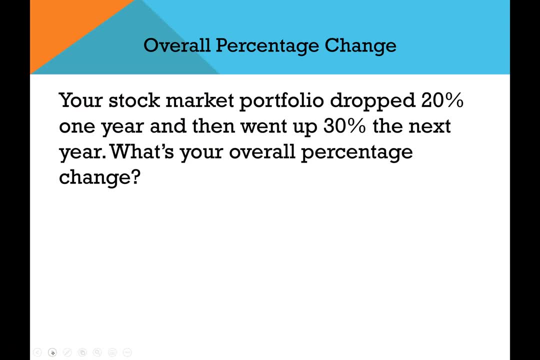 up 15.5% And that's because you're taking 10% of a bigger number here. All right, Let's talk about dropping and then going back up. So stock market portfolio dropped to 20% one year and then went up 30% the next year. What's your overall percentage change? Again, let's start with 100.. 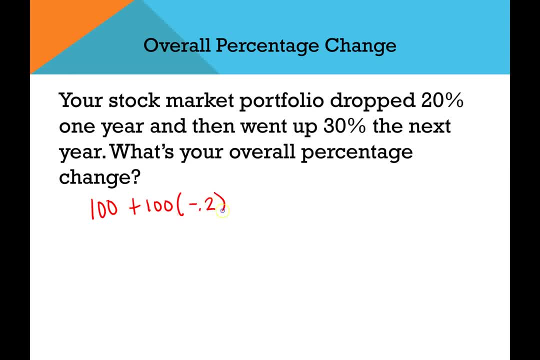 We're dropping negative 0.2.. That's 20%. That's going to give us an $80.. Now we're going to take this $80. And now we're going to go up 30%. Okay, This one I do have to do on my calculator. 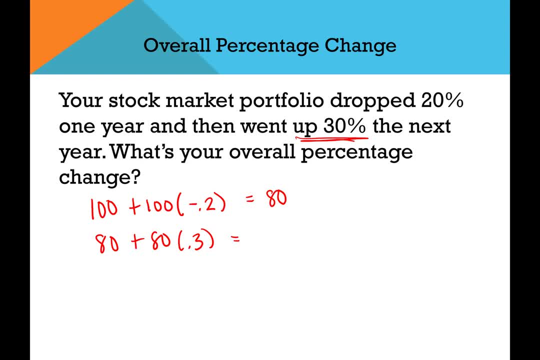 and I get 104.. All right, So let's see if this works. New minus old over new. Well, new minus old. So this is going to be our new value of 104 minus a hundred over a hundred. All right, That's going. 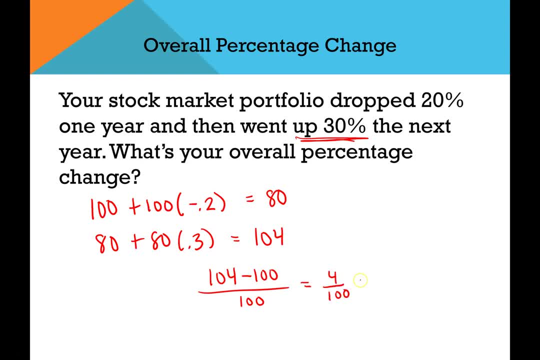 to give me four over a hundred, which is going to be equal to 0.04 multiplied by a hundred, And we do get 4% increase. All right, Well, it looks like we're in pretty good shape to say if this: 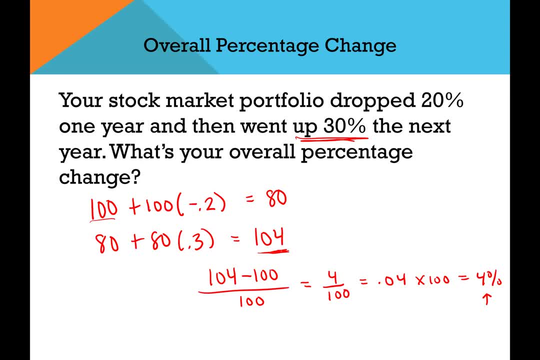 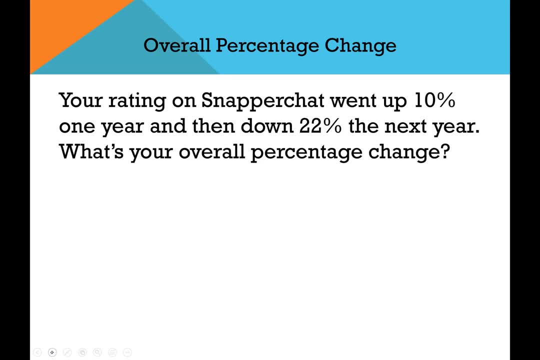 is a hundred and this is 104, we're up 4%, And guess what? That's why I chose a hundred. All right, Let's take a look at this one. Your rating on snapper chat went up 10% one year and 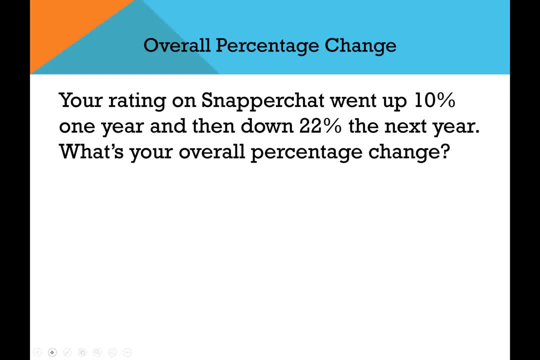 down 22% the next year. What's your overall percentage change? This one feels like we're going to get an answer that is going to be down. So maybe this pattern won't work with the hundred and the 104.. Let's see about that. So, starting with a score of 100 and then going up, we're going to. 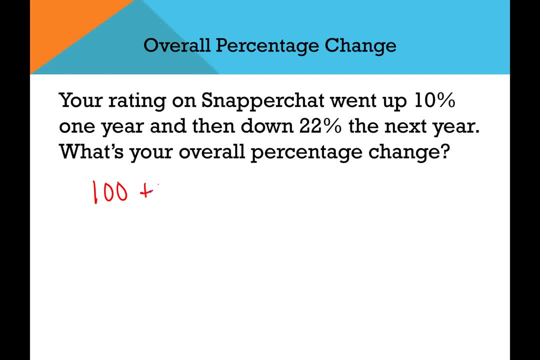 go up, Oops, 100 plus 100 times 0.10.. That's going to give us 110.. Then we're going to have 110 plus a 110 and then a negative 0.22.. So that's going to give me one second, folks. I get 85.8.. So in a case, 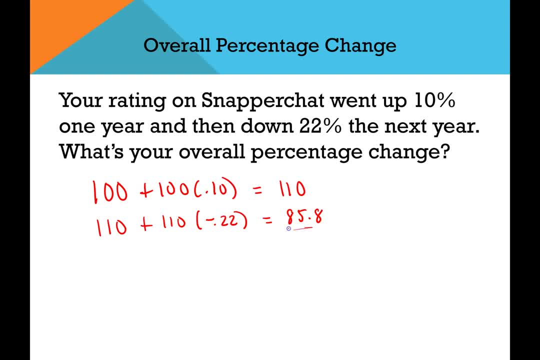 like this: I'm going to get a negative 0.22.. So I'm going to get a negative 0.22.. So I'm going to guess we can't just simply say it went up by blah blah blah percent, but because actually it went. 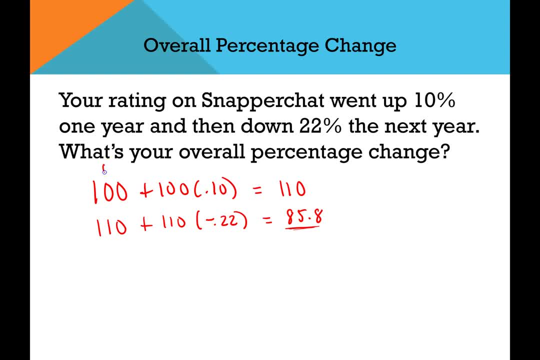 down. So this is my old value. This is my new value. So we're going to do new minus old over old. So that's going to be my new, which is 85.8 minus my old, all over my old. So this is going to. 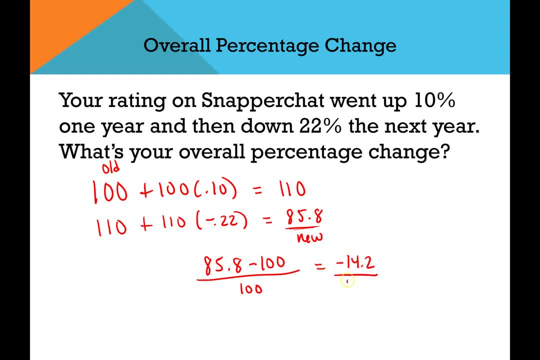 give me negative 14.2 divided by a hundred. Okay, That brings my decimal over two. I get negative 0.142 and multiply by a hundred and we get a 14.2%, But this time a decrease, right, Because of the.